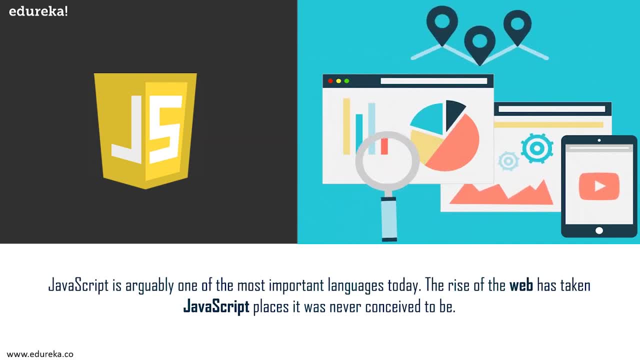 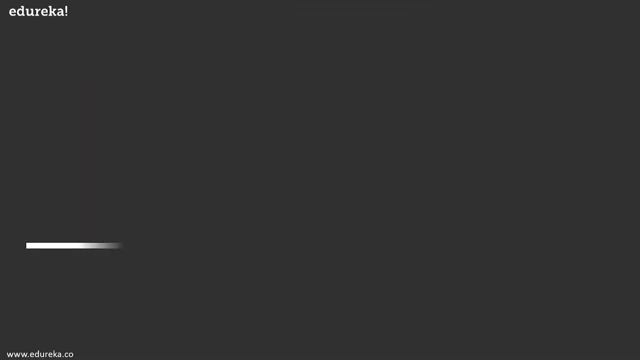 So if you want your web page to look alive and do a lot more than just gawk at you, JavaScript is a must. Now there are certain basic concepts and fundamentals that you must know before you begin to write a code in JavaScript. So these fundamentals of JavaScript includes the variables: 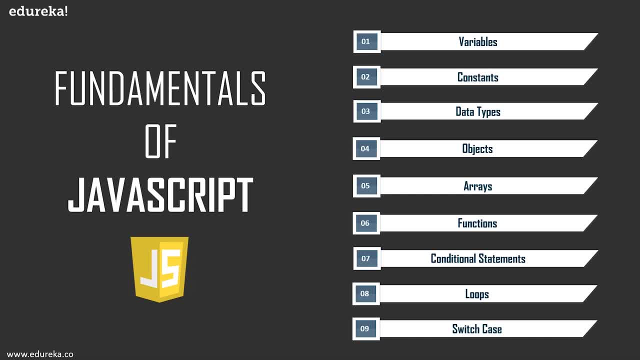 constants, data types, objects, arrays, functions, conditional statements, loops and switch case. in today's session, We will be discussing one of these fundamentals, that is, the functions in JavaScript. Now you can go back and check out our videos on JavaScript tutorial- What is JavaScript? and also learn JavaScript. 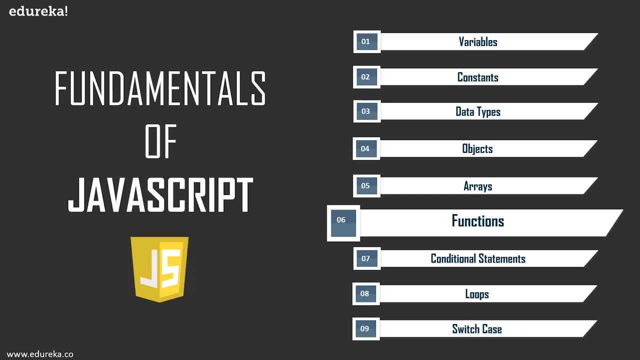 in 60 minutes in order to get a detailed description about all of these fundamentals and also if you want to know more about how JavaScript works, you can go back and check out those videos. But in today's session we will only focus on the JavaScript functions. 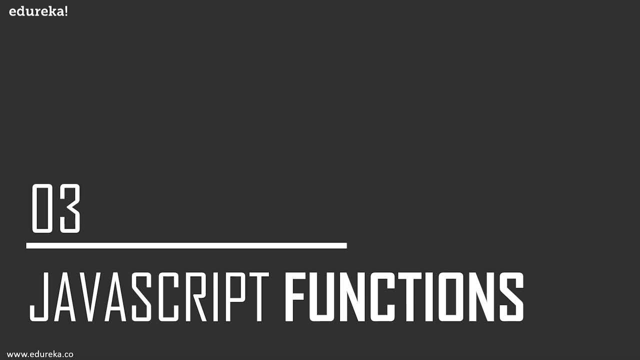 How are they defined in JavaScript and how do they actually work now? A JavaScript function is basically a block of code that is designed to perform any particular task, So you can execute a function by calling it. this is also known as invoking or calling a function. now to use a function. 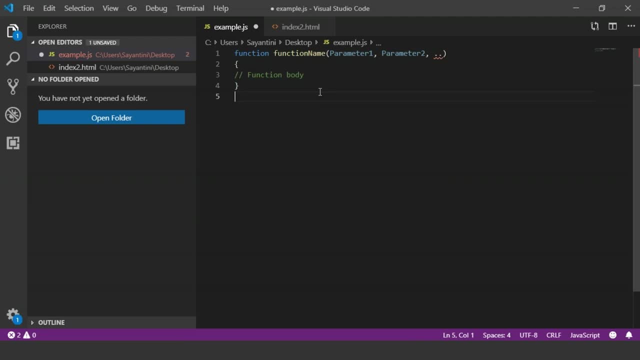 You have to define it somewhere in the scope from which you wish to call it. the ideas is to put some commonly performed task together and make a function so that, instead of writing the same code again and again for different inputs, We can call that particular function. 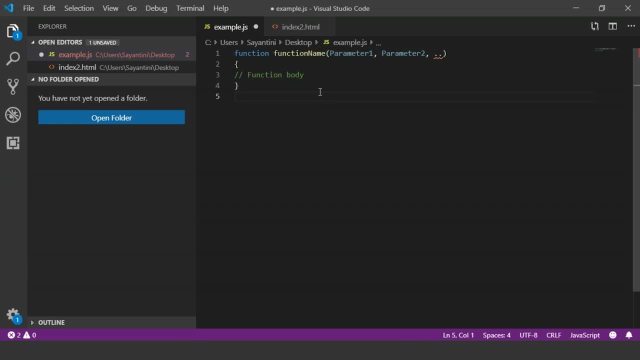 So let's see how you can define the function in JavaScript. So let's have a look at the basic syntax. So first we have the keyword as function, after that We specify our function name here and here you can declare your parameters that you want to pass through your function. 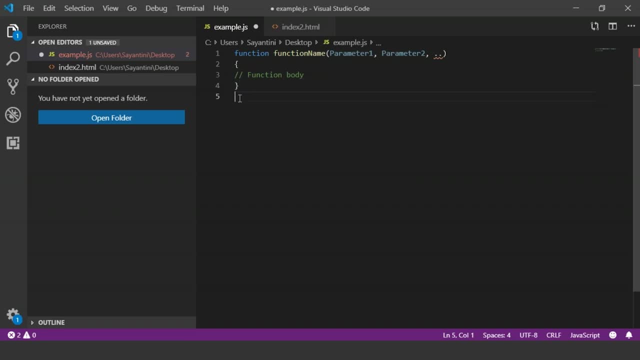 And then finally, here you will have your function body and then later on you will be calling that particular function. So let's see how this works. So let me just take the square of a number. So, for example, I want to name my function name as square. 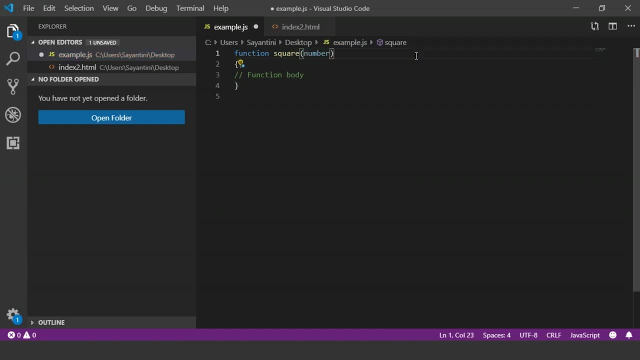 and I am. I'm passing the parameter as number here. Now, here I have declared my function name and inside this I've passed the parameter as number. now, here I have to give the return value as well. So what this is going to return me is number into number. 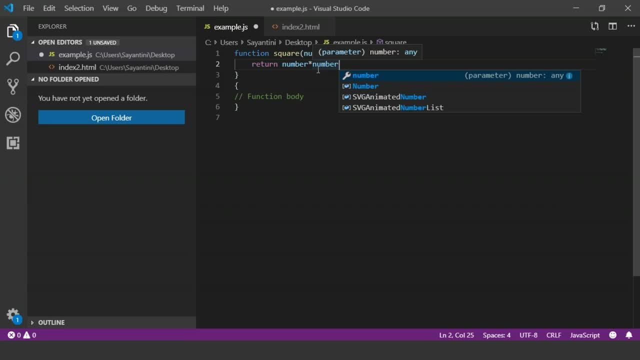 This means the number into number- will return me the value of the square of that particular number. now here I'll Define the number as number equals to square of. suppose we are taking any particular number. For example, I'm taking the number to be for now. 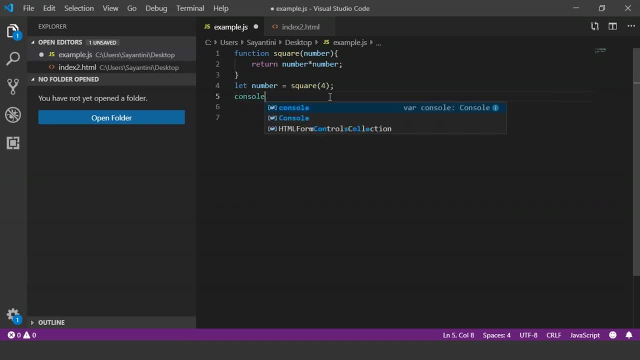 Once I have taken the number as for, I will take the console Dot log as number. So now here, what happens is I have declared the function as square, inside that I've passed a parameter. Now I want to return the value as number into number. 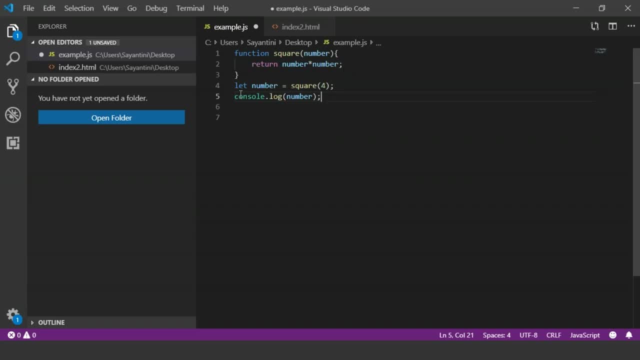 which will give me the square of that particular value. So now, in the function body, we have defined the number as square of 4.. Now, finally, I have to print the value here now in order to get this particular value, that is, the square of the number 4.. 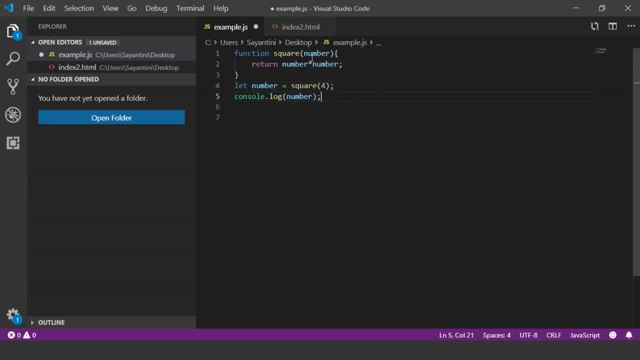 We have to print the number. So basically, we are calling the parameter that we have defined inside our function squared here. So now let me just save this one. Now, when we go to our console, you can see that the output shown here is as 16.. 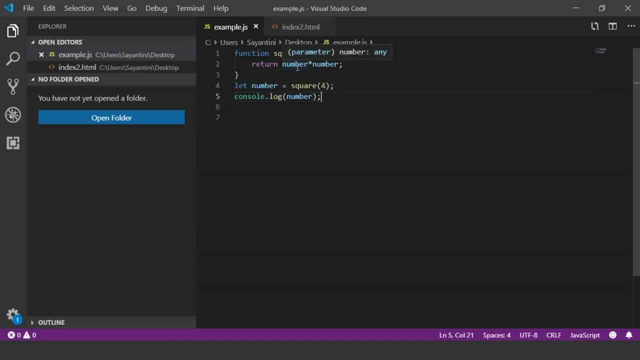 So what happens is that it takes the number as 4, returns the value as 4 x 4, that is, the square of this particular number, and prints the value to be 16.. So this is how a function works. Now, for example. 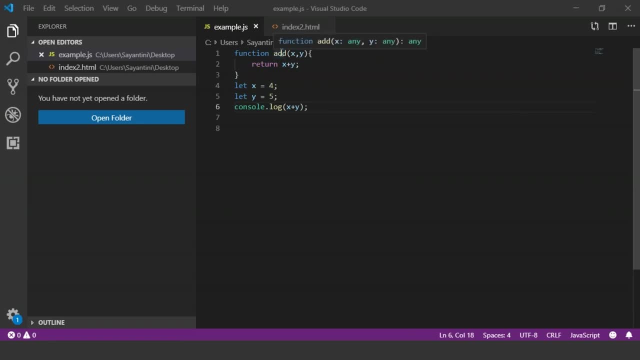 if you want to add two numbers, you can use your function name as add. So here we have: the function name is add and I'm passing the parameters as X, comma, Y. Suppose I'm taking two different numbers as X and Y. So here, what is the return value? the return value would be: 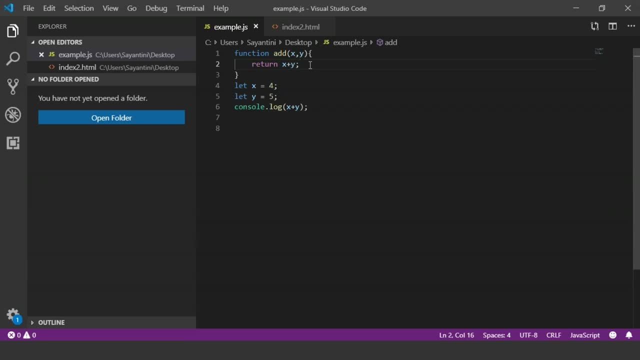 X plus Y, that is, we want to have the sum of these two numbers. So now, once this is done, we will go to the function body and define the values. So here I have given the value of X as 4 and the value of Y as 5.. 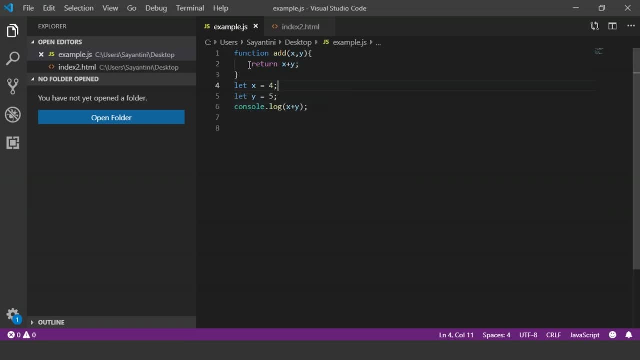 So now, in order to get the value as 9, we need to get the return value as X plus Y. So we will write console dot log: X plus Y. So this will return the value here of our function add, where we have defined two parameters. 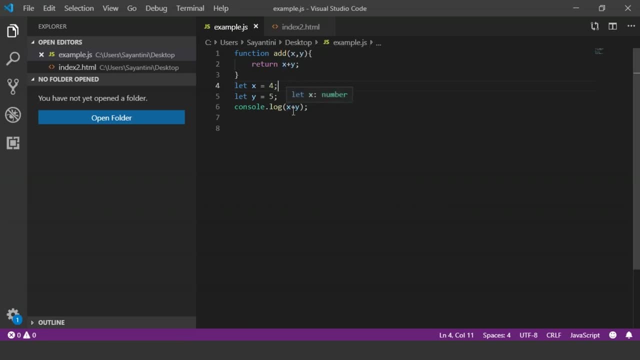 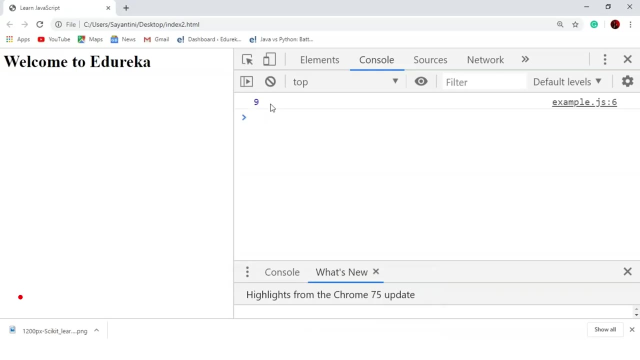 as X and Y, and it will add both of these numbers and give me the output. So now let me just save this, and then when we go to our console, you can see that the output declared here is 9.. So this basically gives me the sum of my two values. 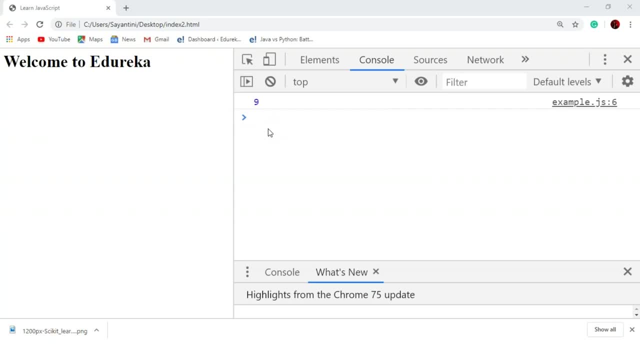 or the two parameters that have passed in my function, That is, X and Y, where the values are 4 and 5, and it has given me the sum as 9.. Now, these are the different user-defined functions that you can use, or you can name your function in a particular manner. 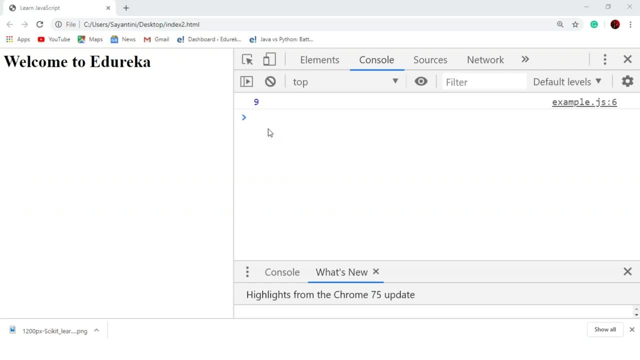 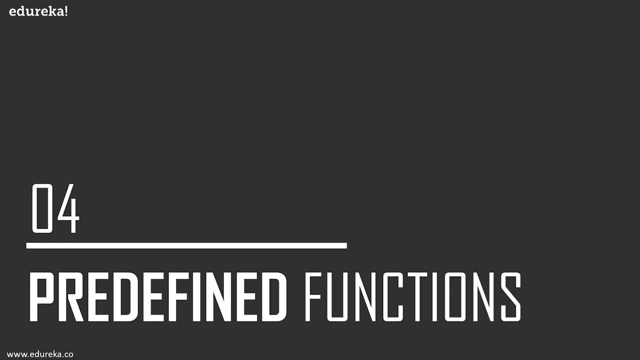 where you can understand that, what you are trying to do- and you can create any function of your own, but there are also loads of predefined and built-in functions in JavaScript, So let's have a look at some of the most important or some of the oldest predefined functions. 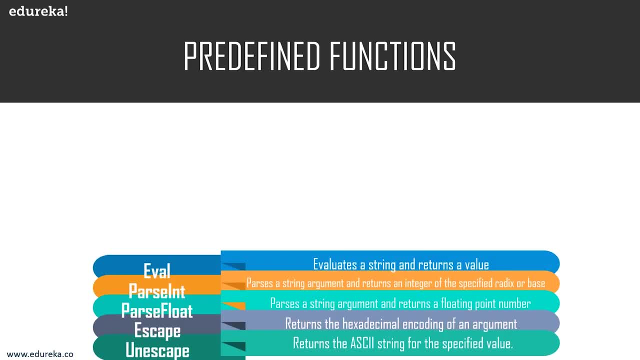 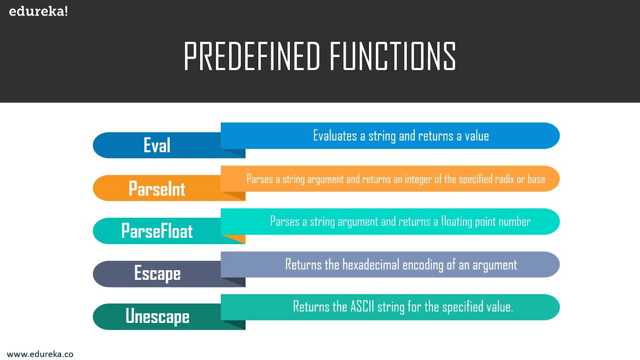 that were built into the language itself. Now, JavaScript has several top-level built-in functions, but there are five functions that are built into the language, and those are the eval, parseInt, parseFloat, escape and unescape. Now, what does the eval function do? 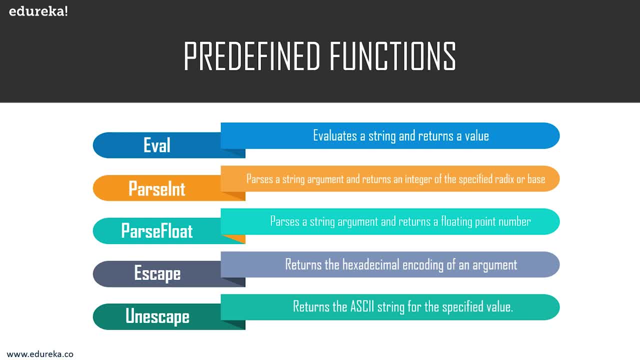 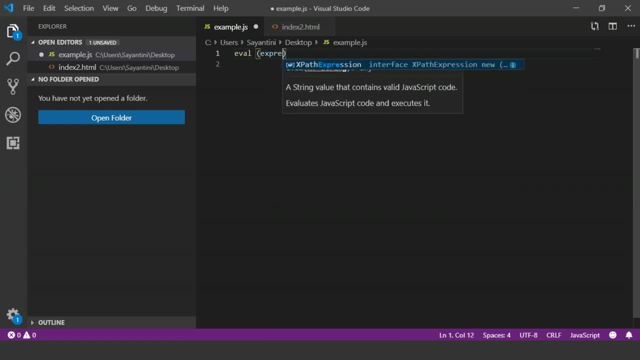 Now this will evaluate a string and also return a particular value. So for your eval function, you just need the function as eval and inside this you have to pass your expression. You can put on any expression here. Now this expression will be evaluated and if the result is not a string, the result is returned. 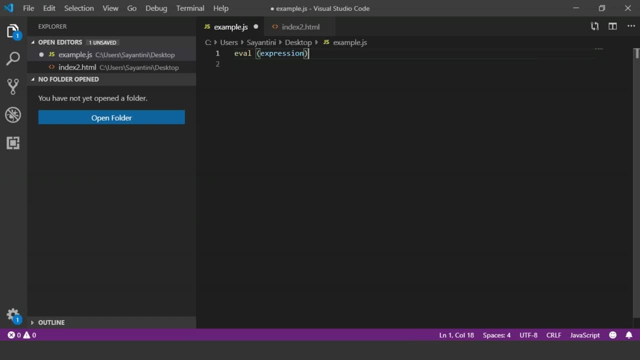 and in case the result is a string, it is taken to be a JavaScript program and then it is evaluated. Now, if the program completes, normally, eval returns the value of the last expression in it. Now, for example, let me take these variables as let x equals to 2. 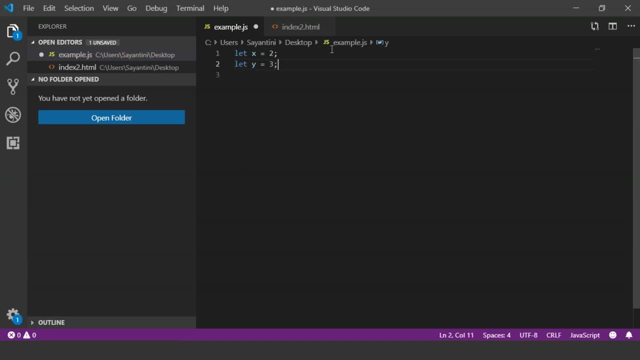 then let y equals to 3 and then here I will have my eval function. So I'll just take console Dot log eval and I will just take the values of my x and y as a string. So I'll just write x plus y. 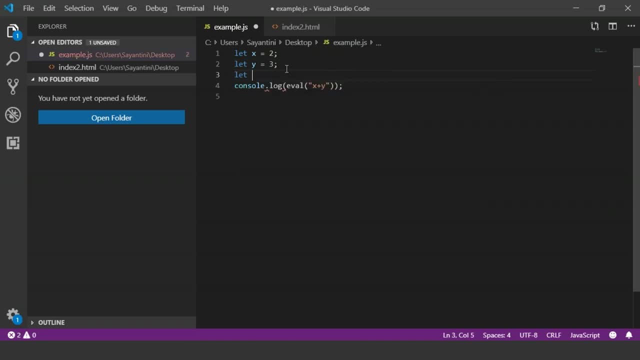 Now here let me just define another variable as Z, So Z equals to 4. and then in the next one I will just take it in the format as it is, that is, console Dot log eval zed. So now let's save this one. 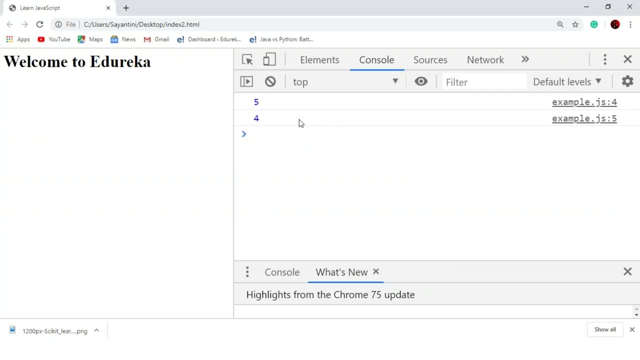 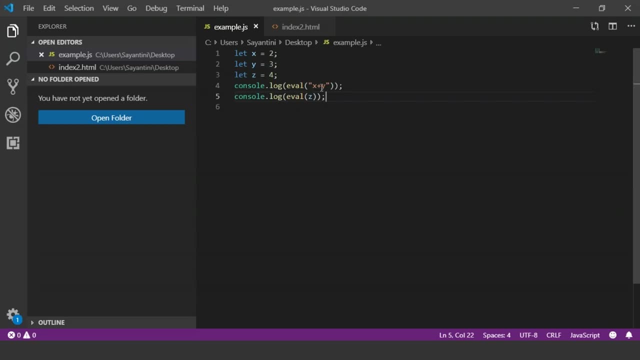 So now, when we go back to our console, you can see that we have two outputs. The first one is 5 and the second one is 4.. So what happens here is that in the first one it takes the value as string. 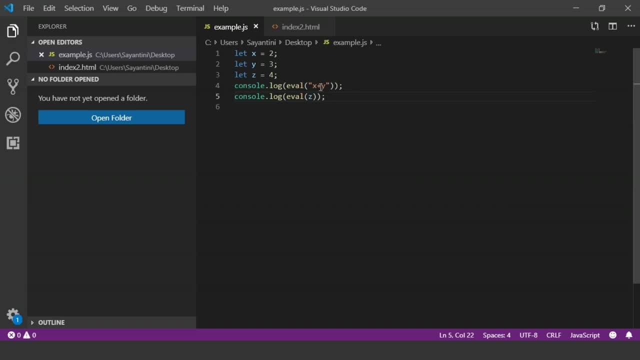 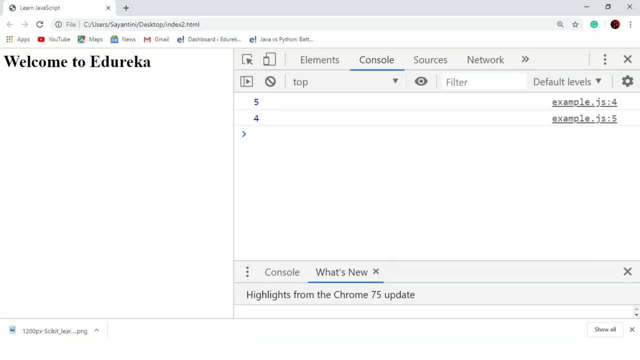 but it will return the value as it is. So we have x plus y as 2 plus 3, that is, the value is 2 plus 3 equals to 5, and we are getting the output as 5 here and in the next one. 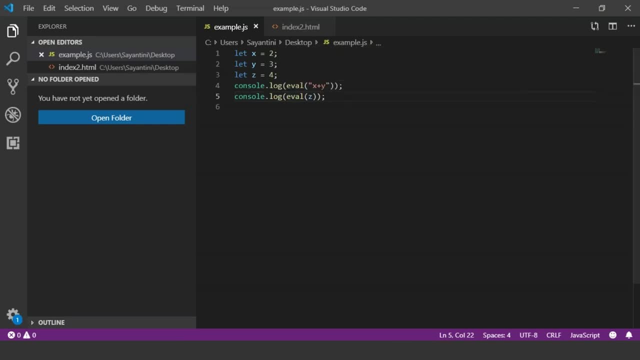 it will give me just the value of Z that I have defined here. So what happens here Is that when you have a string inside your expression, it will evaluate the values inside the string and then return the value. That's exactly what happened here. 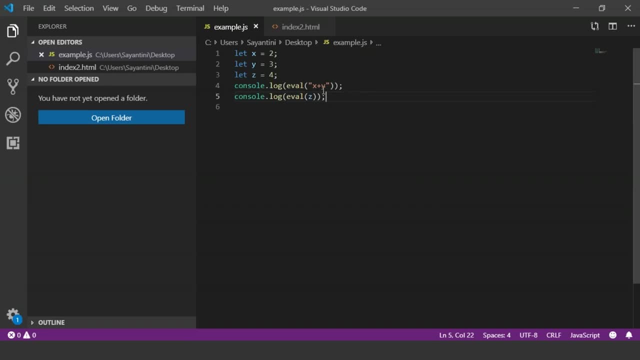 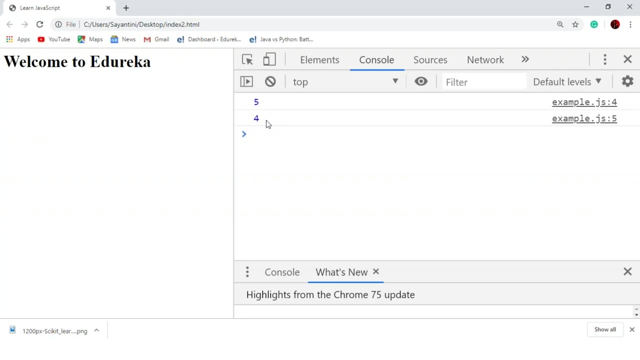 Even though we took x and y as strings here. it evaluated the values for both x and y, that is, 2 plus 3, and gave me the value as 5 and in the second one and return me the value as it is, because it was not defined as a string or anything. 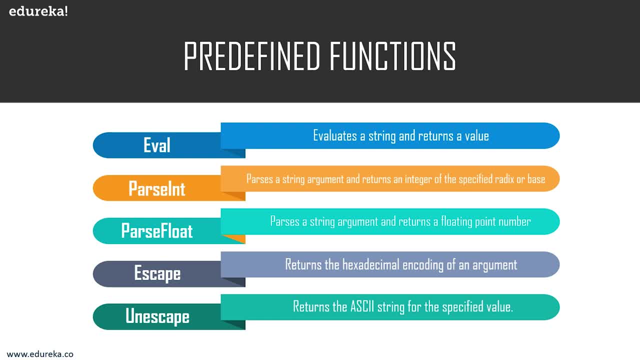 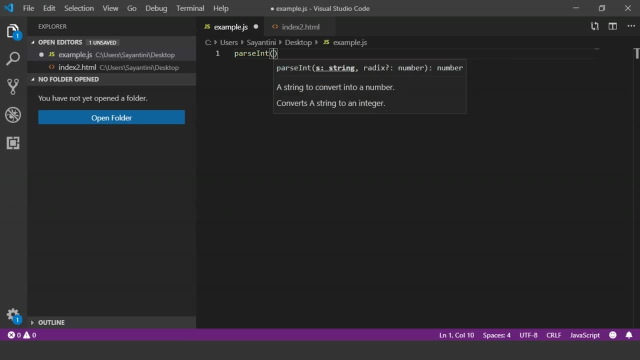 Now the next one is the parse int. now the parse int function basically parses a string argument and returns an integer of the specified radix or base. So for parse int all you have to do is just write parse int function inside this. You just have to define the parameter. 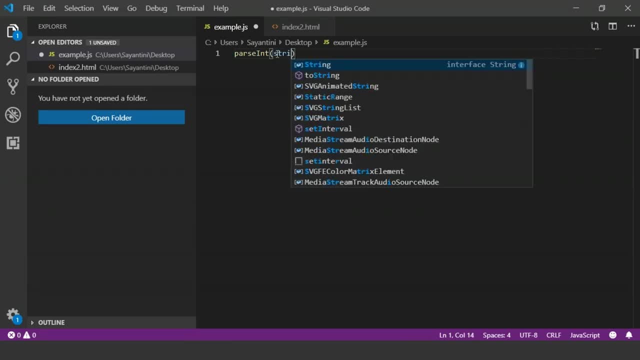 as whatever you are passing here, So whatever string you want to pass here, will be inside your parse int. So what it does is it will take the value and convert it into the radix or base value. Now, next up is the parse float. So what parse float? 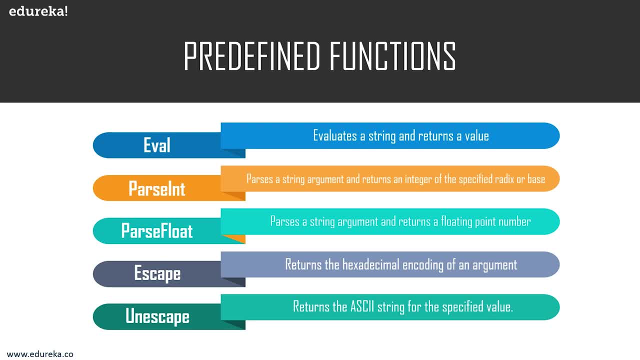 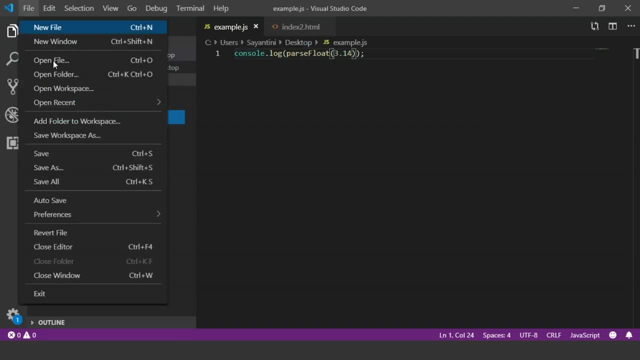 Does it. it passes a string argument and then returns a floating point number. Now the syntax is very simple: You just have to write parse float and then pass your string inside your parameters. So here we have an example as consolelog: parse float 3.14.. 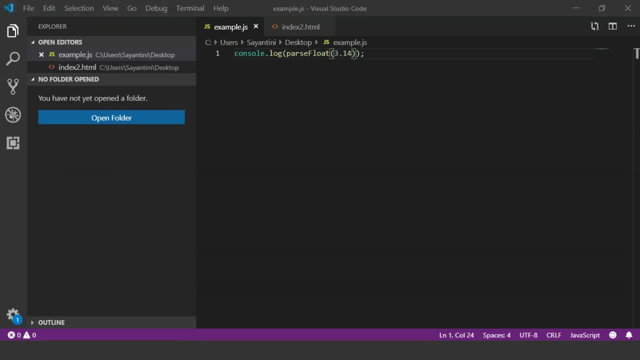 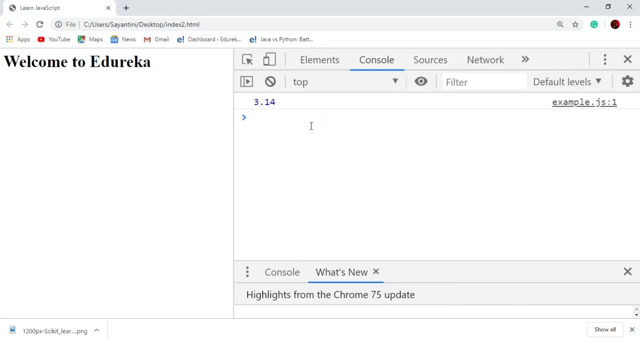 So here we have a floating number, So I will save this, and this will return me the value in the form of a float. So it takes any particular string and then passes the float value of that particular number or that particular string itself. Next up we have the escape. 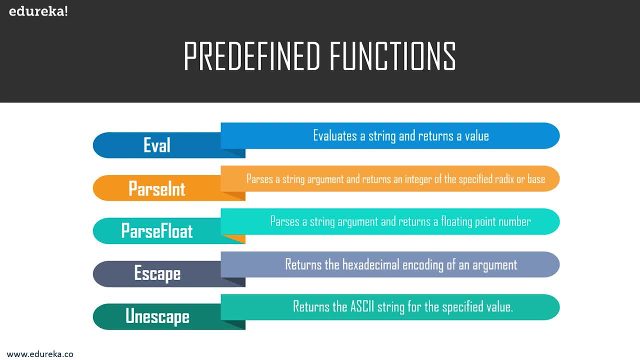 Now, escape returns the hexadecimal encoding of an argument in the ISO Latin one character set. So all you have to do is just take the escape function and pass your string inside this. Now the value returned by the escape function is either for the alphanumeric characters or for the space character. 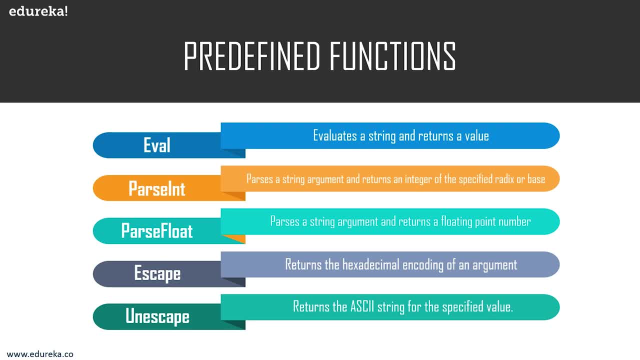 or the plus sign, and for alphanumeric characters other than the space as well. and next up, we have the unescape function. now, unescape function returns the ascii string for the specified value, So it's similar to the escape function. All you have to do is just write an escape function. 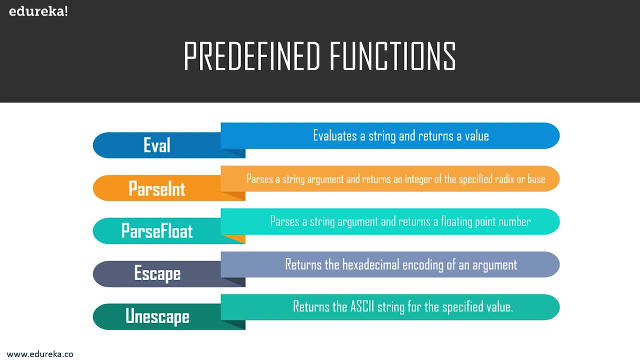 and pass your string inside it. Now the unescape returns the corresponding ascii character in the ISO Latin one character set. So these were some of the predefined functions. There are many more top-level predefined or built-in functions in JavaScript that you can use while writing. 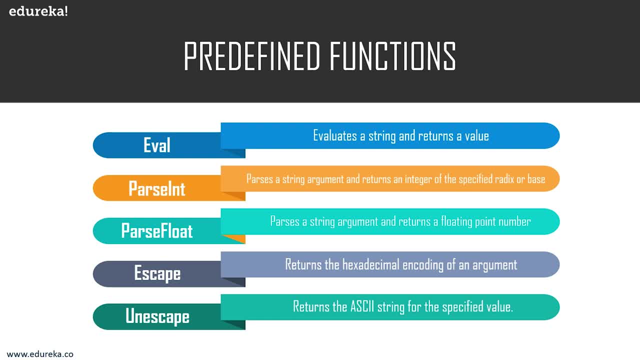 on any particular code in JavaScript. So you have the constructor to fixed to string, value of, to source, and all of these built-in functions that are already there, with the help of which you can define any particular string, or you can take any parameter and perform your function in your JavaScript code. 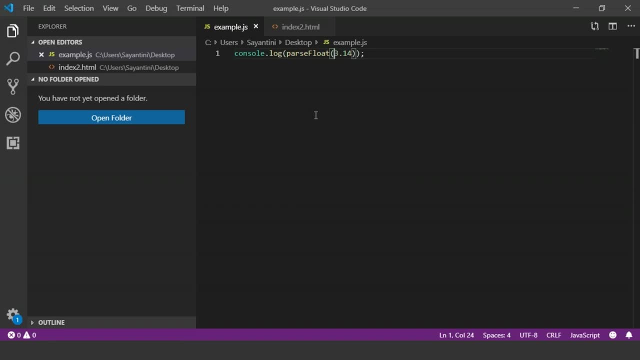 So we have already discussed about the different predefined and built-in functions and, as we all know, we can create our own function. that is, you have the option for the user defined functions in JavaScript, which makes your work easier. You can just create a function with a name. 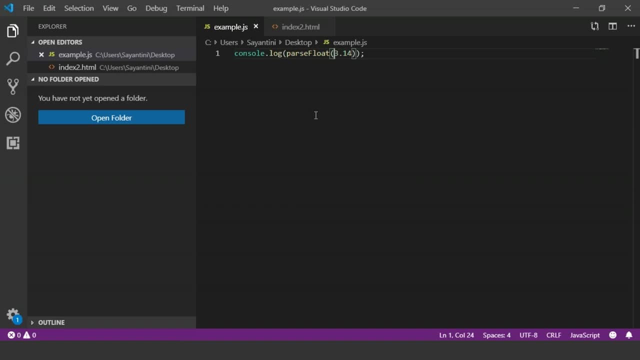 that is suitable for whatever function you're going to perform, like for addition of two numbers. You can give the function name as some, or add or something like that, which will make it easier to understand that what that function is trying to do. So now let's move on. 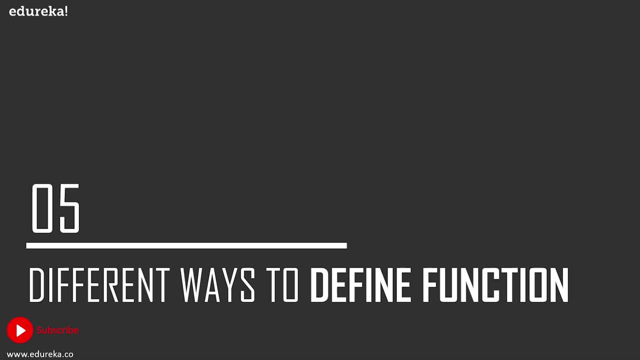 and have a look at the different ways to define a function. Now, a function is a parametric block of code defined one time and called any number of times later. So in JavaScript, a function can be declared using several ways. talking about the first one, 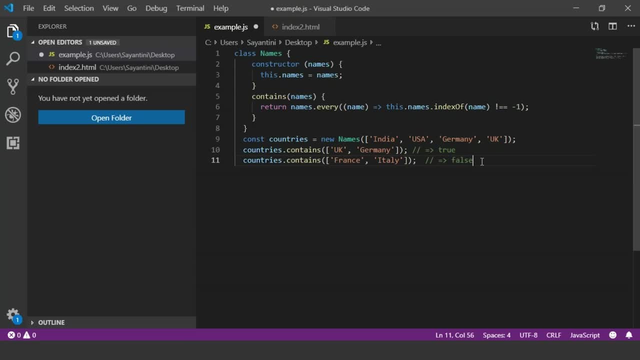 We have the function declaration now. the function code has a slight impact on what declaration type to choose, but it is important to know that how the function interacts with the external components and the invocation type. now the arrow function passed to the dot. Every function has this, that is, the instance of names class. 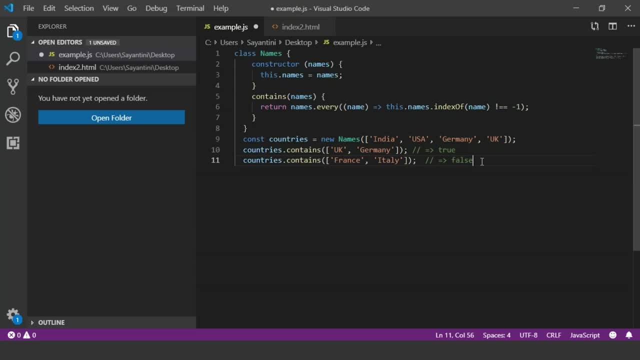 now the same as contains method. a function declared with the fat arrow is the most appropriate declaration type in a case when the context needs to be inherited from the outer method. that is, the dot contains function. Now, if you're trying to use a function expression for the dot, every function callback. 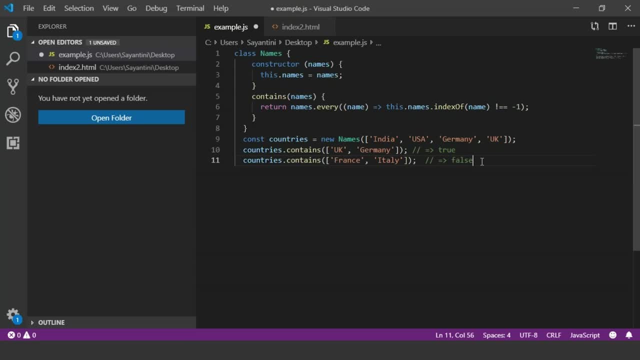 it would require more manual configuration of the context. So this was just an example on how functions can work in JavaScript. So there are different methods in which you can define these functions. The first one is the function declaration. So let's have a look at an example for function declaration. 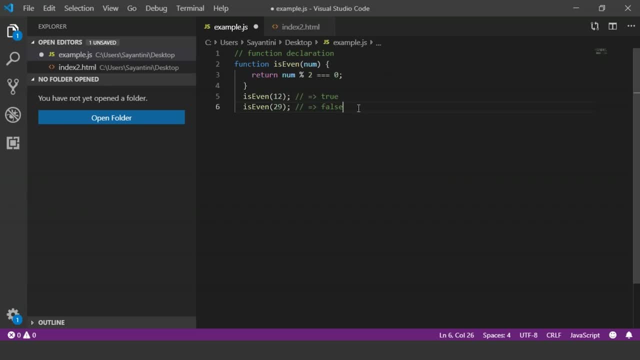 So here we have an example that shows how we can declare the function or how this function declaration works. now, here the function is even. num is a function declaration that defines: is even function, which determines that if a number Is even or not, now the function declaration usually creates: 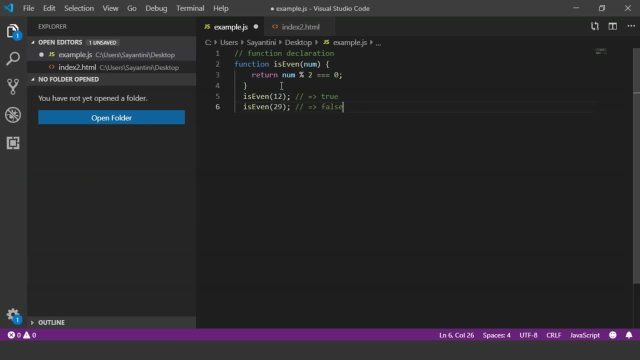 a variable in the current scope with the identifier equal to the function name. Now this variable holds the function object. So what happens here is that the function variable is hosted up to the top of the current scope, which means that the function can be invoked. 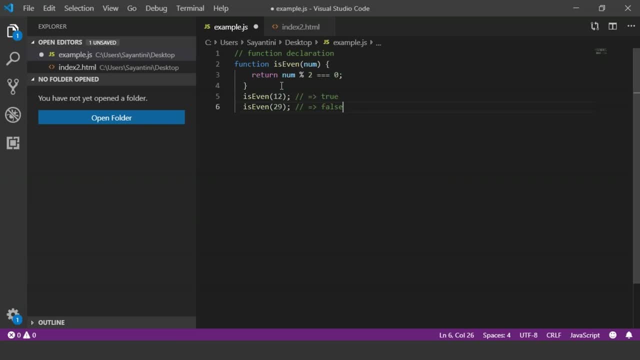 before the declaration itself. So the created function is named, which means that name property of the function object holds its name. So it is useful when viewing the call stack in debugging or error messages reading. So what happens here is that I have the function is even num. 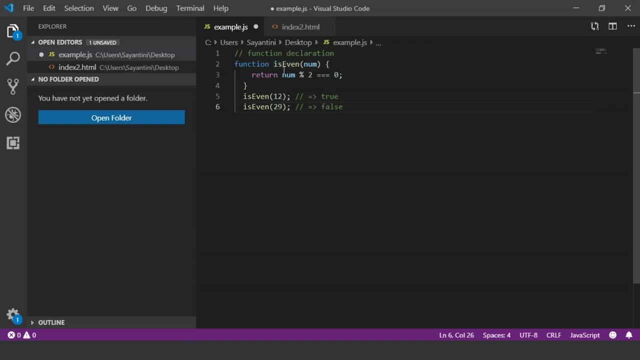 and then I have returned the value as num. person to equal equals zero. So what happens here is that it will give me the value that are only even. so any number that is even is also divided by 2.. So here I have given two numbers as 12 and 29.. 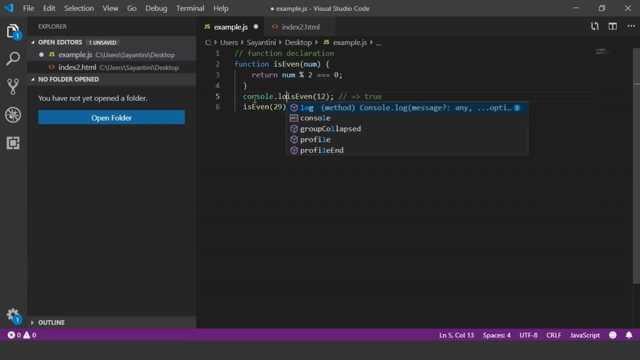 So when I take the print for these, suppose I have console dot log and is even the number is 12, and the same I do for the number 29 and just give console dot log here. So what happens is that 12 modulus 2 would give me the value. 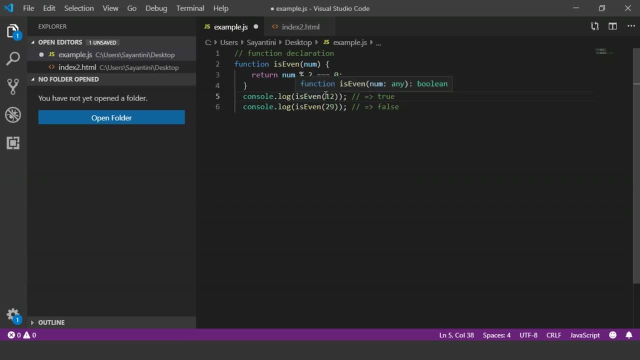 as 0, but 29 modulus 2 won't. so this is an even number. So the output would be true and this is not an even number, So it will return me the value as false. So now let me just save this. and now when we go back to our console, 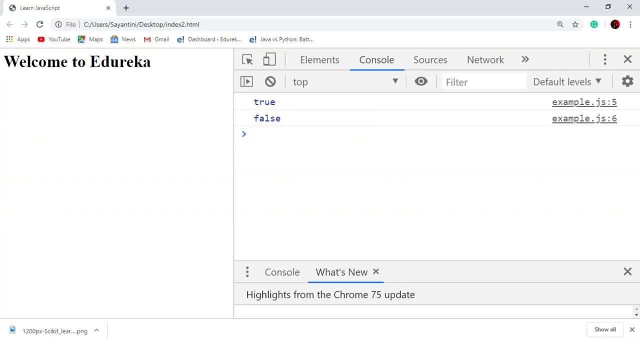 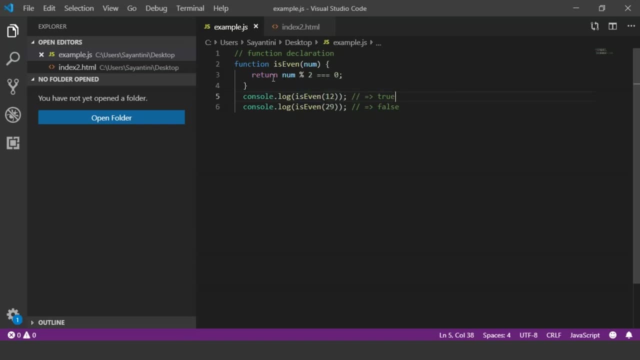 you can see that we have the two outputs as true and false. So for the first number I have got the output as true, because it is definitely an even number, and here I want to return the value where the number modulus 2 gives me the value as 0. 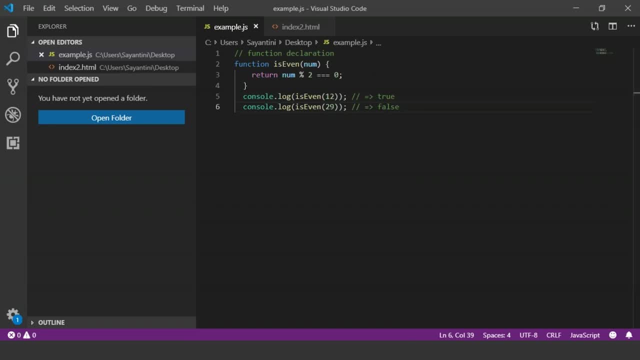 and for the second one, it definitely prints as false. Now let me just take another example for the factorial. So here I have the factorial function and inside this function a recursive call is being made Using the variable that holds the function. So here I have factorial n minus 1. now it is possible. 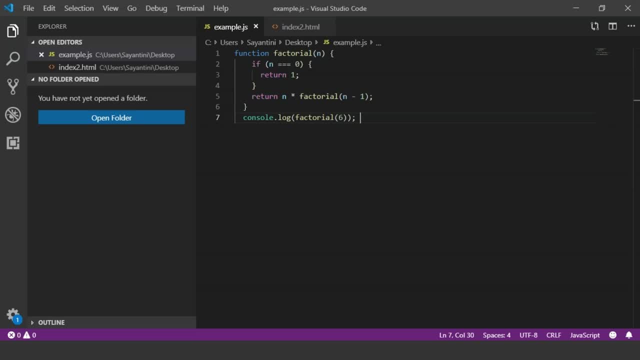 to use a function expression and assign it to a regular variable. that is suppose we can write as let: factorial equals to factorial n, but the function declaration, that is the function factorial n, looks more compact. So we don't need any variable or any let keyword to define it. again and again now. 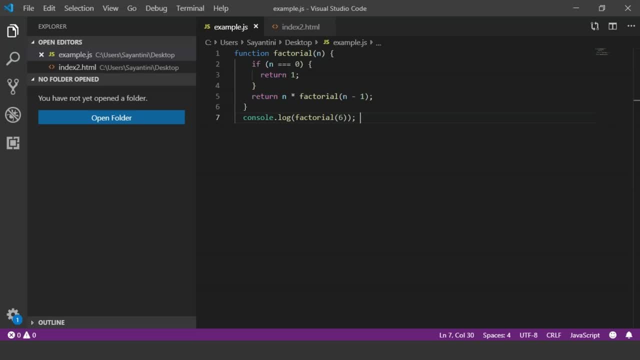 an important property of the function declaration is its hosting mechanism. So here what happens is that we have the function declaration as function factorial n and inside this, directly, We have returned the value as 1 if n is equal to equal to 0. So here I'll just take the factorial formula. 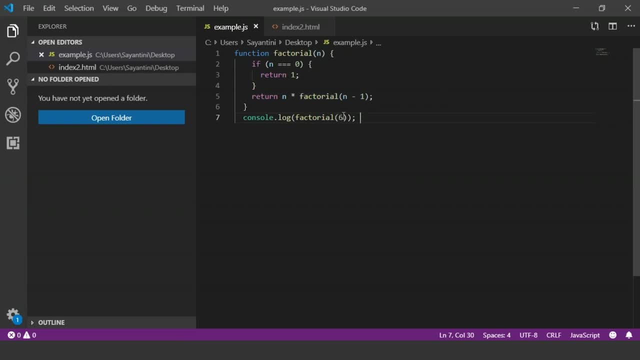 that is, n into factorial, into n minus 1.. Now let me just take any value for which I want to find the factorial. So I have taken the number as 6 now let's save this one Now when I go back to my console. 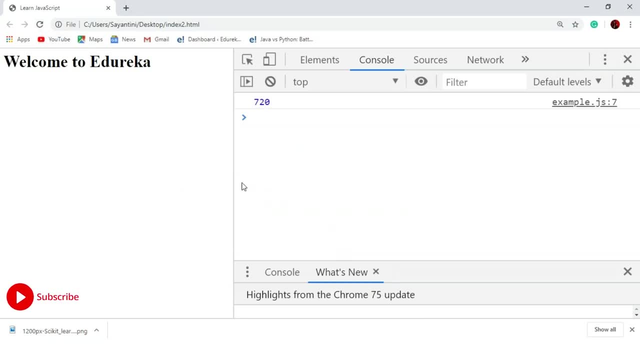 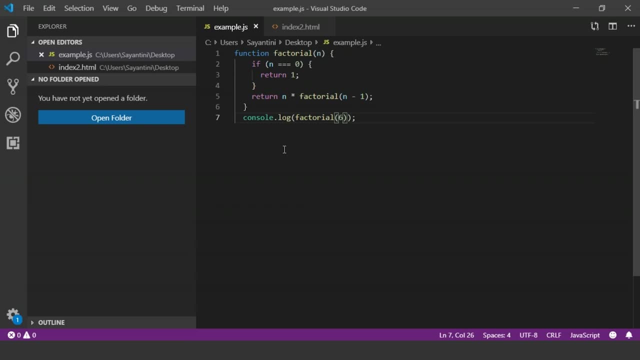 you can see that the output is 720.. So this gives me the factorial value for 6 here. So this is how easy it is when you use the function declaration here. So this was just one of the methods to do this. next up: 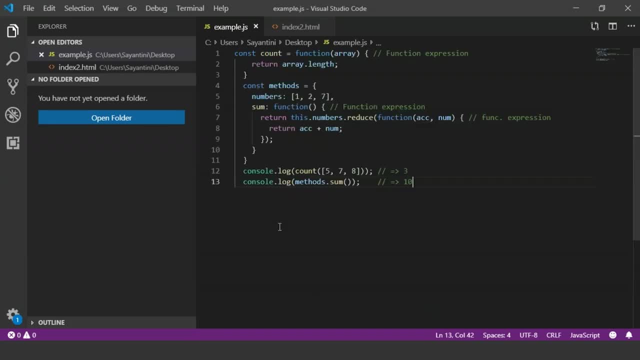 We will have a look at the function expression Now. a function expression is determined by a function keyword, followed by an optional function name. Now a list of parameters in a pair of parentheses and also a pair of curly braces that delimits The body code. now all of these together. 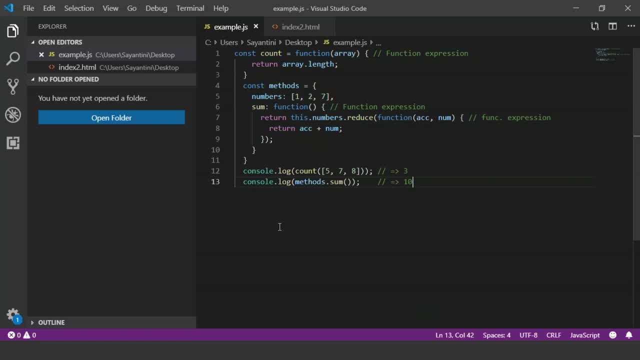 make up your function expression. So here we have an example for the function expression. So this expression creates a function object that can be used in different situations. So first it is assigned to a variable as an object that is, count equals to function, and then we have given the values. 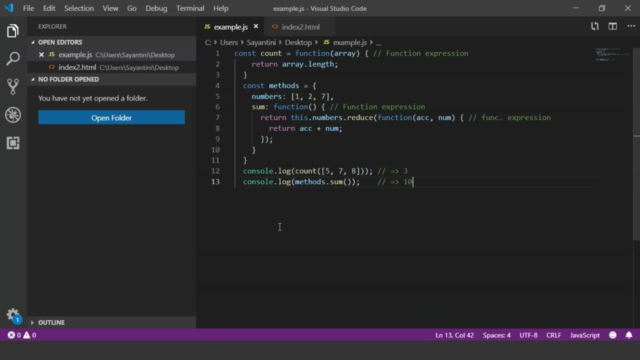 and next, we have used it to create a method on an object where we have used the sum colon function. So this is used in order to find the sum of the values. and finally, we have used it for the function as a callback where we have the dot reduce function as well. 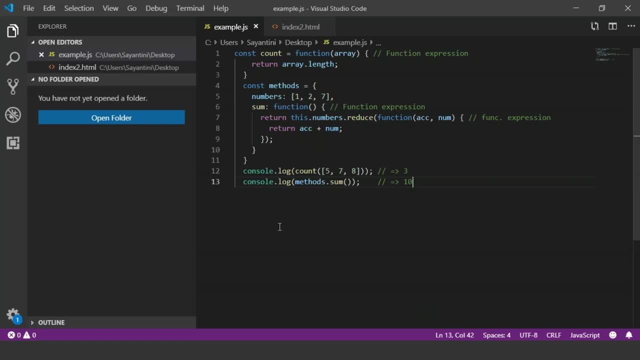 Now the function expression is the working horse in JavaScript. most of the time developer deals with this type of function declaration alongside the arrow function. now, looking at the code, You can see that first we have declared the constant count equals to function array and we have returned the array length. 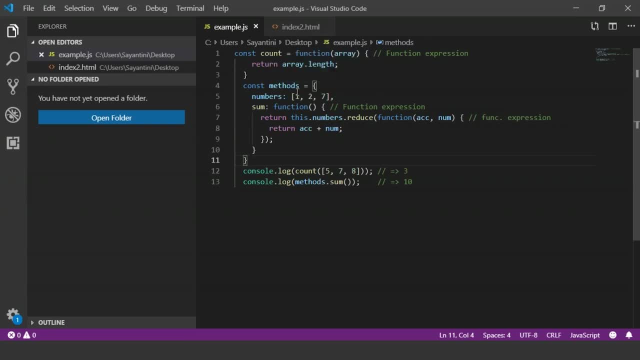 So now here this is our function expression. So now, inside this, we have our methods, Where we have defined the numbers as 1, 2 and 7, for which we are going to find the sum, and we have passed the same function expression here as well. 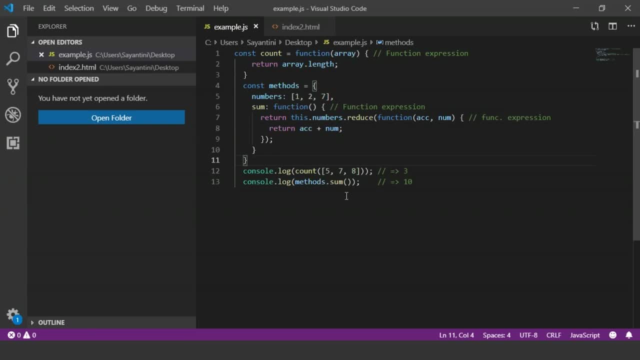 So now, if I want to get the output, as first I want to count the numbers that are there, that is, I'm using this particular count function here, and then next up I want to see the sum of the methods that I have defined here. So I will just take consolelog count, suppose. 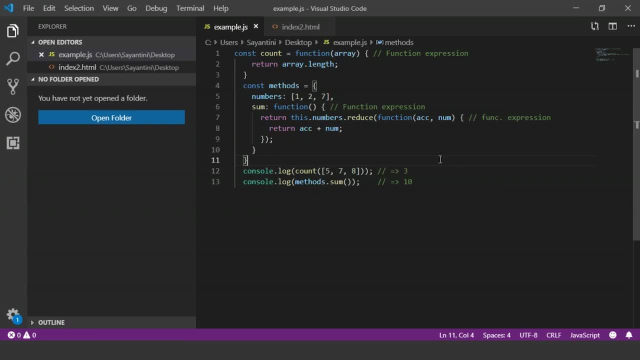 I'm giving any three numbers like five, six, seven, eight, So it should give me the count to be three. then I have taken the methods dot sum function where I'm going to take these particular numbers, that is, 1, 2 and 7, that I have defined here. 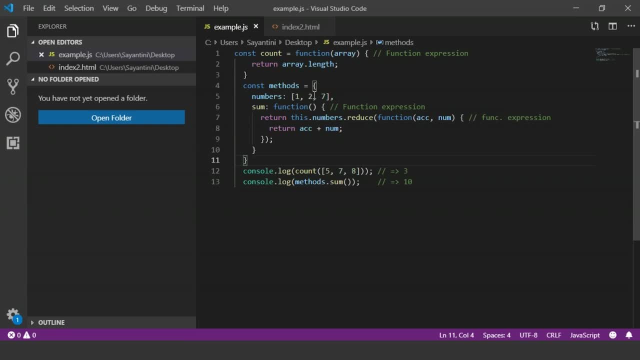 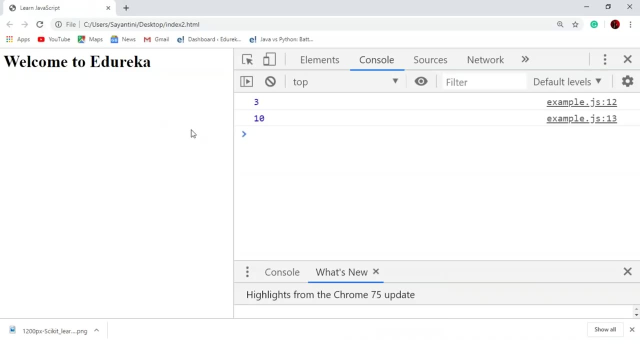 and it should give me the summation. So basically, it should give me the value as 1 plus 2 plus 7, that is 10.. So now, if I save this and go to my console, you can see the output as 3 and 10.. 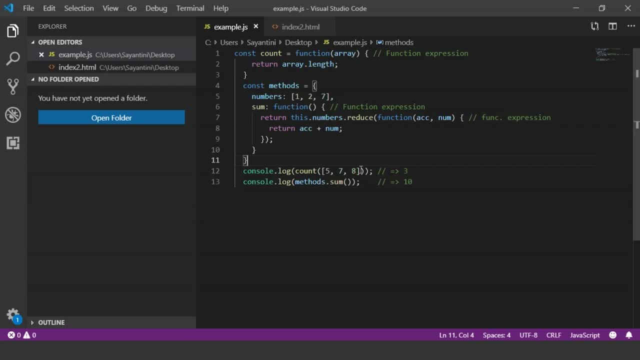 So for the first one it returns me the value of the number or the length, that is, the array length. So here I have three values inside my array, So it gives me the output as 3, that is, it returns me the array length, that is, we have returned the array length here. 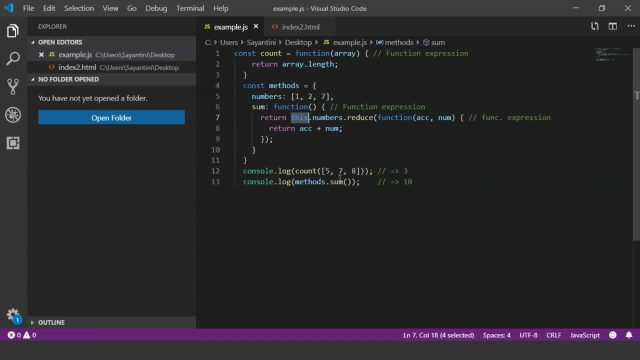 Now in the second one it returns me the sum of this methods dot sum function. So here I have the values as 1, 2 and 7 inside the array, So the total gives me as 10.. So I've got the output as 10 here. 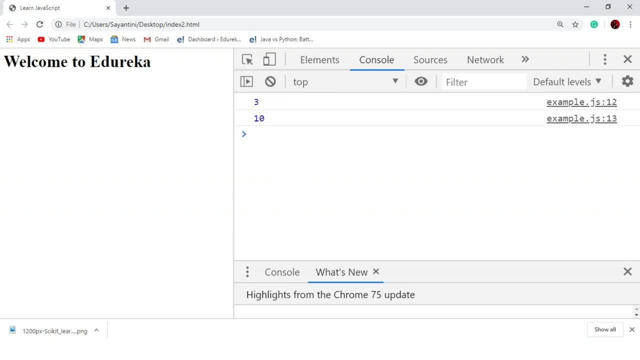 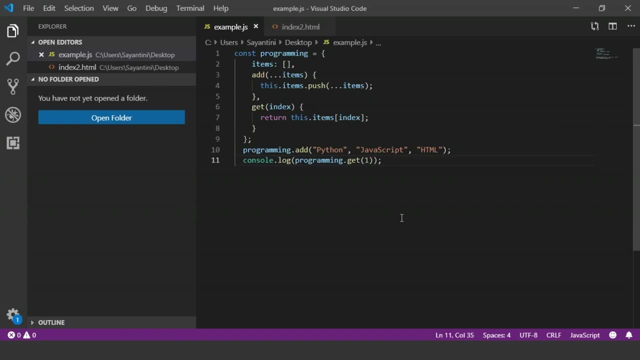 So this is how the function expression works in JavaScript. Now the next one is the shorthand method definition. So here is an example now, before looking into the example. the shorthand method definition can be used in a method declaration on object literals and the es6 classes. 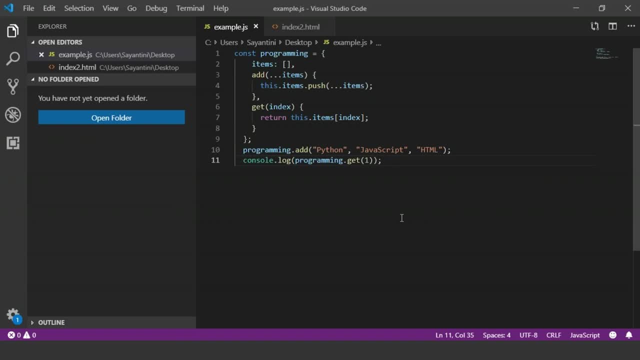 So you can define them using a function name followed by a list of parameters in a pair of parentheses and also a pair of curly braces that delimits the body statements. now, in this example, we have used the shorthand method definition in an object literal, So here we have the add. 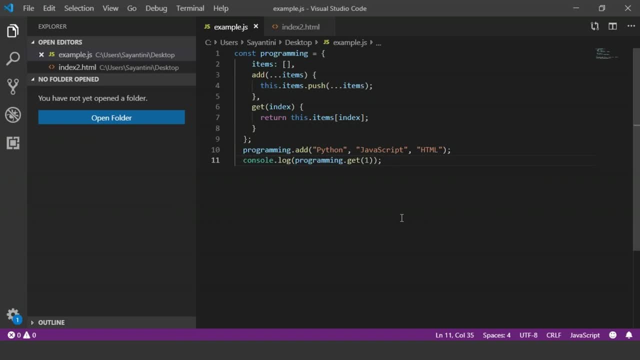 and get methods in our programming object and are defined using the shorthand method definition. Now these methods are called as usual here. So we have our programming dot add and then we have programming dot get method as well. Now the short approach of method definition has several benefits over traditional property definition. 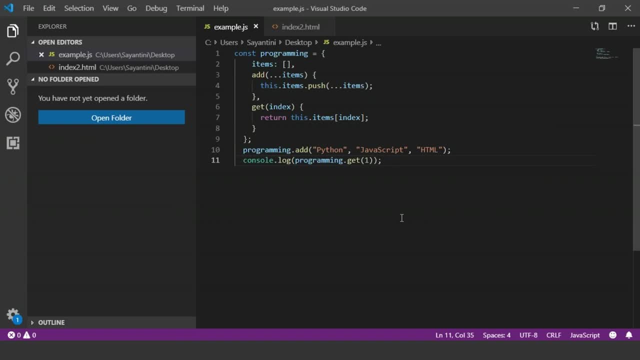 Basically it gives you a shorter syntax that is easier to read and write and also shorthand method definition creates named functions contrary to a function expression. It is also very useful for debugging. So in this example you can see that we have the constant as programming. 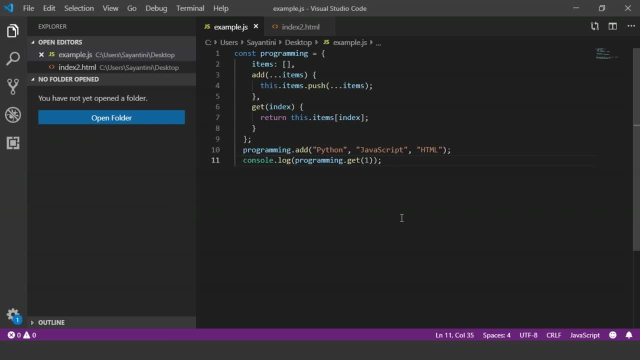 and in this we have added items, that is, we have pushed items inside this and also got the index value as well. So, basically, we have created the array with the index value and we have pushed the items inside it too. So now, in order to push this- items inside this- 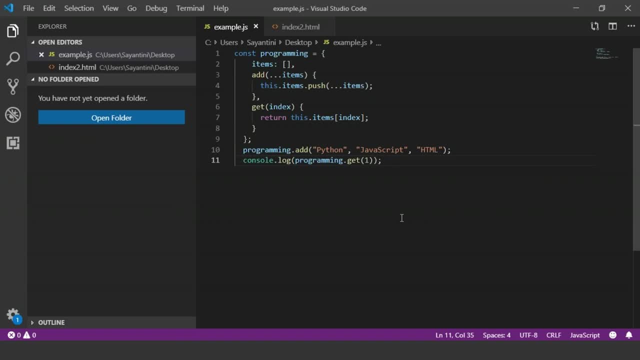 what we will do is. so here for my add method. I have added these programming languages- Python, JavaScript and HTML. Now, if I want to get these items with the help of the index value, So what I can do is here I have the get index method that I've used here. 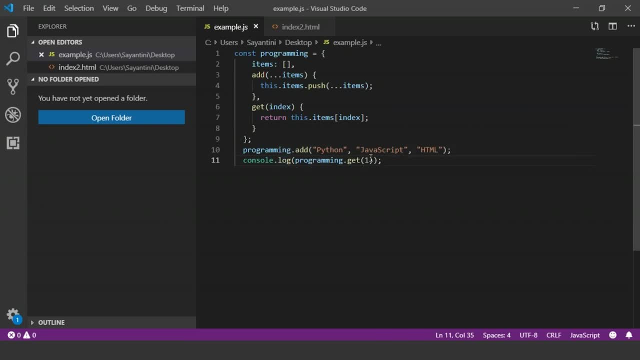 So I'm going to take the output as programming dot get and give the index value. So here I've given the index value as one. So in this particular area the index value one belongs to JavaScript. So now, if I save this and go to my console, 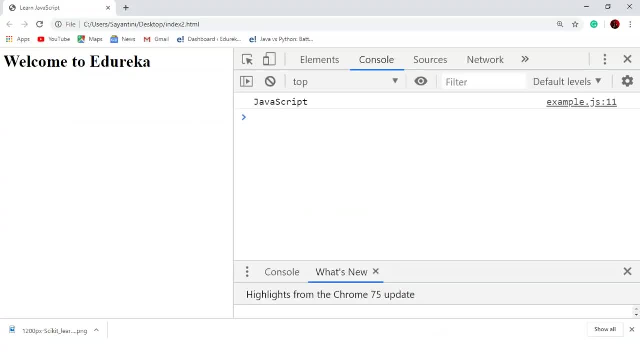 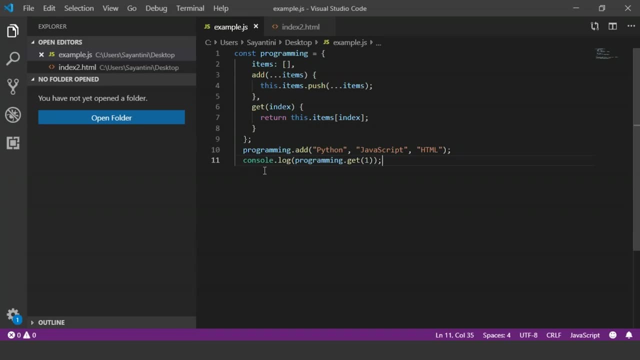 you can see that the output is taken as JavaScript. So first I have used the add method here and added the list of items inside my array, and then what I have done is taken the get method and then taken the index of any particular item that I want to view in my output. 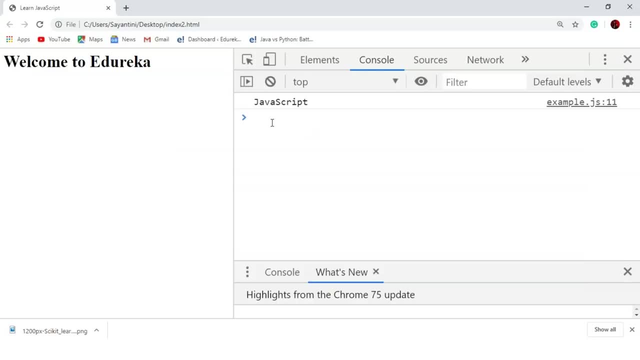 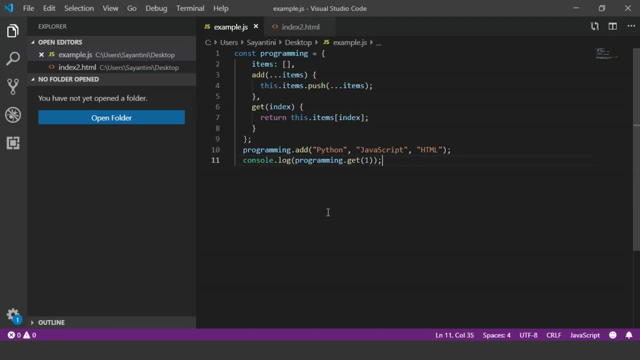 and given that particular index value here. So this is exactly what it gives me the output as. so I have JavaScript because I have given the index value as one here. So this is how the shorthand method works here. Next up, we have another function defining method. 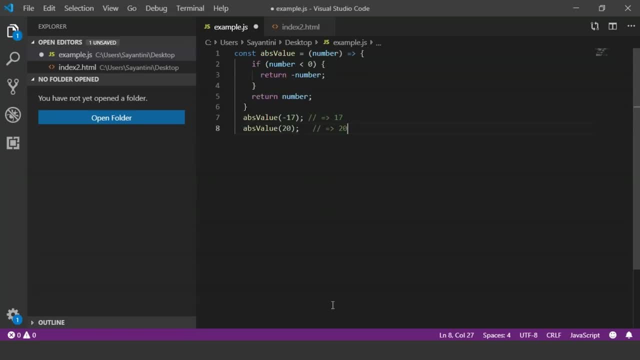 that is the arrow function. now, an arrow function is defined using a pair of parentheses that contains the list of parameters, followed by a fat arrow and a pair of curly braces that delimits the body statements. So this is what we call as the fat arrow here now. 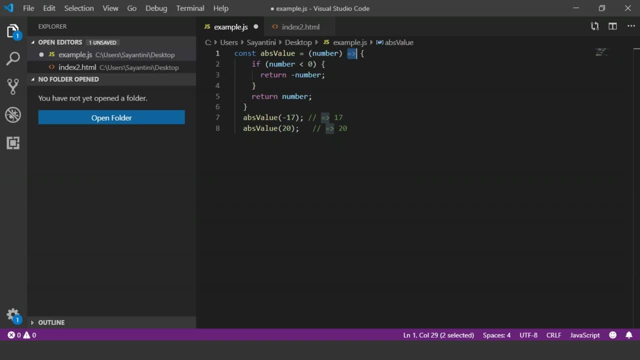 in this example, the absolute value is an arrow function that calculates the absolute value of any particular number. Now the arrow function does not create its own execution context, but takes its lexically. This is definitely an anonymous function, but the browser can infer the functions name. 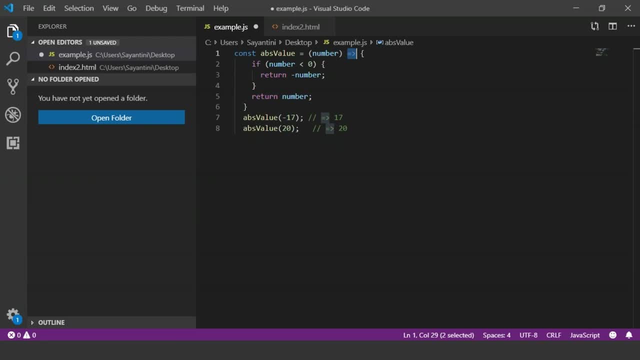 from the variable holding that particular function. object- Now here arguments object- is not available in the arrow function. So what happens here in this example is that it will only return the absolute value for any number that is less than zero. So what happens here is this: if number is less than zero, 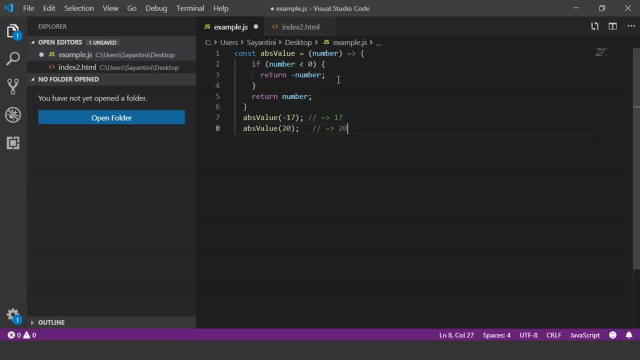 return minus number. So suppose my number is minus 2, it will consider it to be minus minus 2, which makes it a positive number. So basically, any negative number will be taken to be the positive number, That is, the absolute value will be taken. 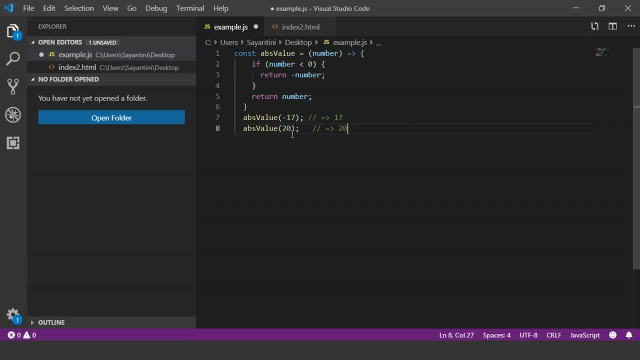 So suppose I have taken two numbers as minus 17 and one is 20. So this minus 17 must be printed as 17.. So let me just take the output. for this I will just take console dot log. Now also for this I will take console dot log. 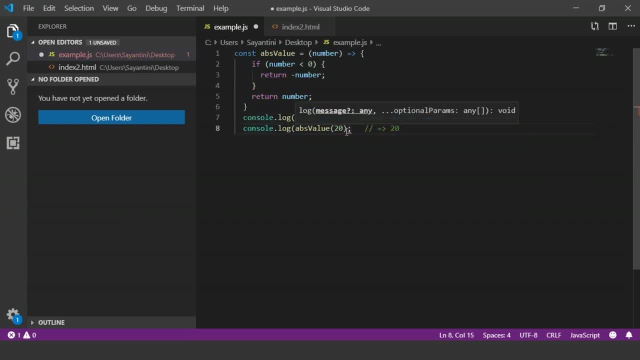 and get the absolute value for 20.. Now, this is already a positive number, So this will give me the same value, But when we have a number less than zero, it will return me the value as minus minus 17,, which will give me 17 as the output. 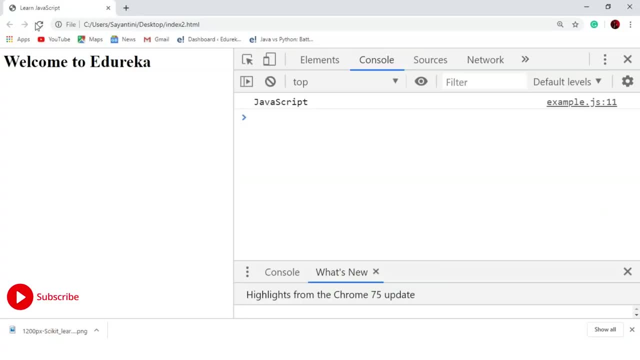 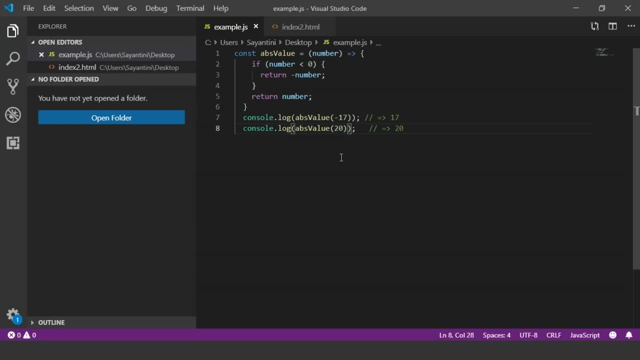 So let's save this. and now go back to the console, So you can see that my output here is 17 and 20.. So in the case of the negative number, it has only given me the absolute value and it has returned the value as positive number. 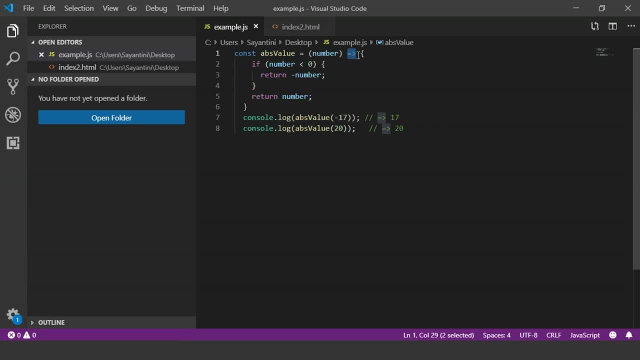 So this is just another use or another way of defining your function with the help of your arrow function. So we have this fat arrow that we have used to define it And finally, we have the generator function. now, the generator function in JavaScript returns a generator object. 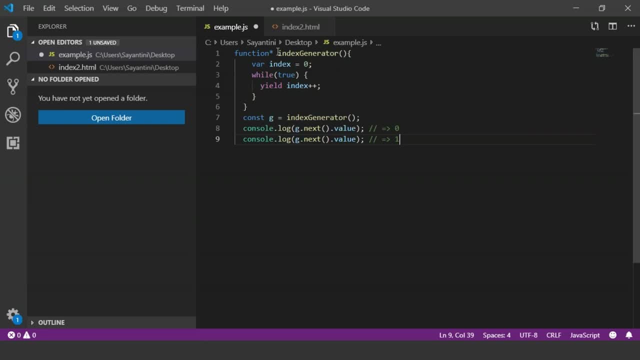 Now it's syntax is similar to the function expression, function declaration or method declaration, just that it requires a star character here. So here we have an example for the generator function. Now this one is for the function declaration form, that is, the function star name. 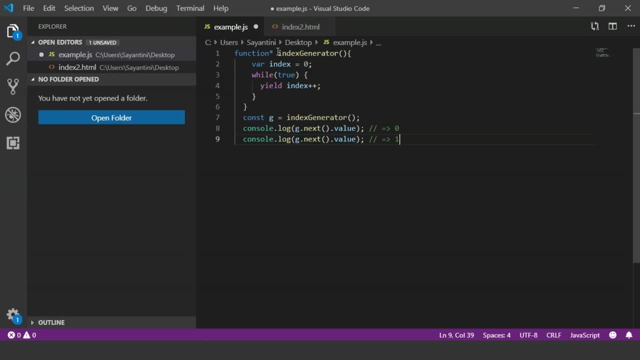 So what happens here is that we have function star index Generator. so you should remember that for your generator function You always need this star character, and here we have to find our index value as 0 and then given the condition as: while true yield index plus, plus. so 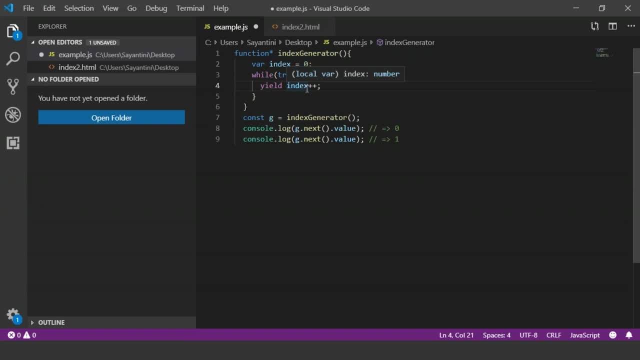 when we have the index value as 0 and then we have index plus plus, that is, it takes up the next value. now here We also need a constant G. So we have our constant G equals to our index generator function. So what we will do here is we will. 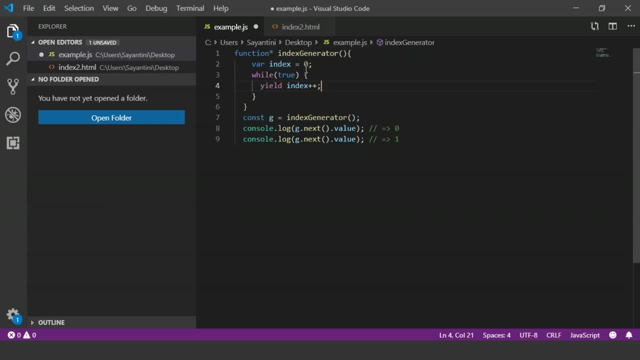 We will take the values first as 0, because we have initialized the index value as 0, and then the value will be incremented here. So the next value that we take is will be 1, because it starts with 0 and then it keeps incrementing. 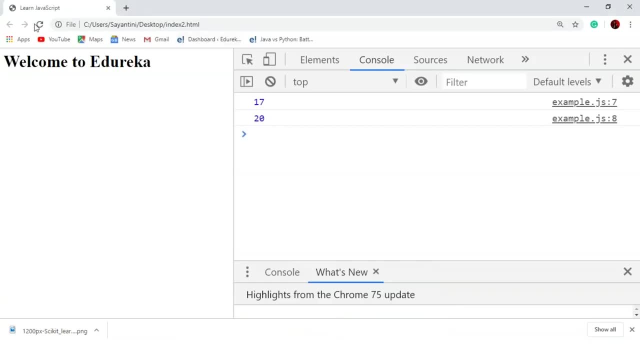 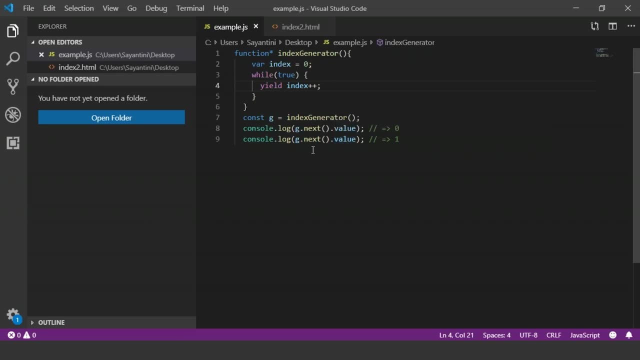 So let me save this And when we go to the console you can see that the output here is 0 and 1.. So if we continue doing this, if we add more G dot, next dot value, it will keep incrementing the value of our index.